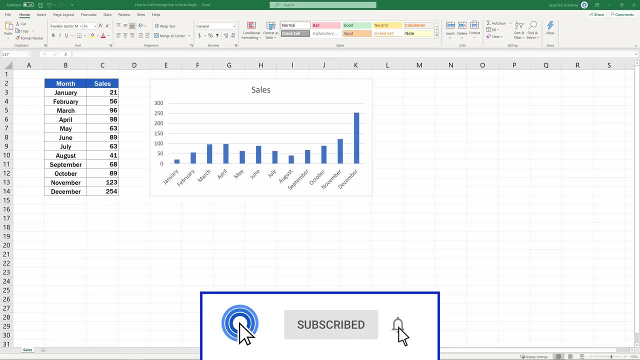 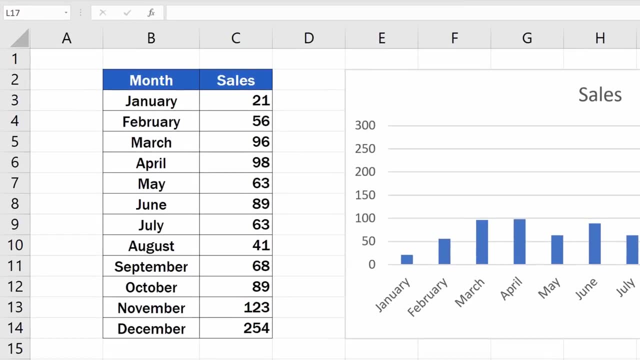 here to make sure you'll be able to use Excel in a quick and easy way, thanks to our digestible video tutorials. If we need to show the average value in a chart, we need to calculate it first. Let's insert a new column right next to the column with sales and name it average. We're also going to adjust. 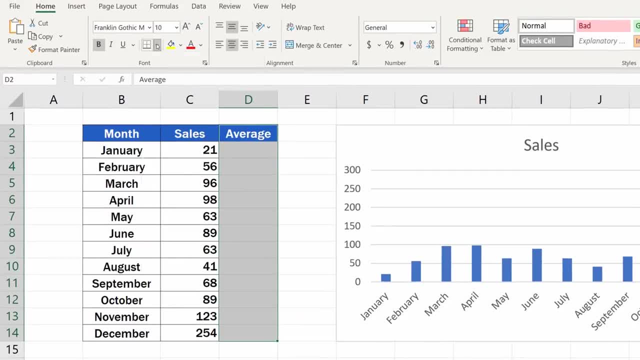 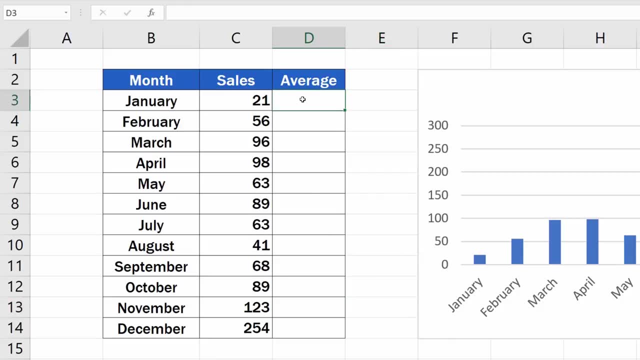 the formatting of the column to make it look like the rest of the table. Great, let's carry on. Click into the first row of the column, average, and calculate the average value by entering the equal sign and typing in average. Click on the suggested function and select all the data from which we're going to calculate the. 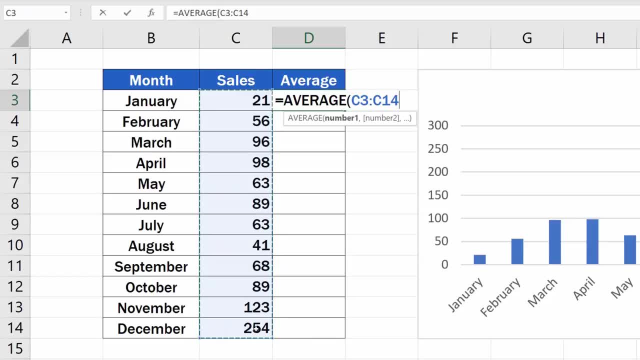 average. Here the range will be all entries in the column sales and we'll close the brackets to see the result. Now we need to copy the function to every row in this column so that the average could appear as a line through every month in the chart. However, if we copy the function as it is, 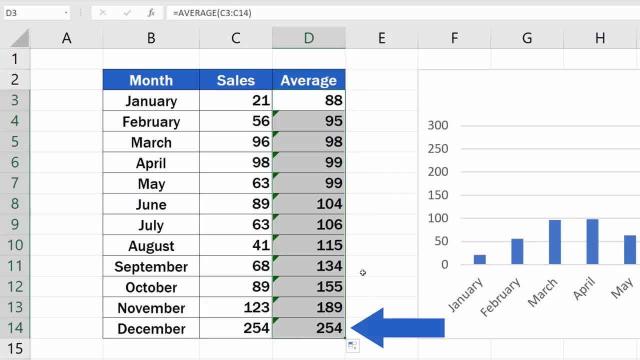 every month shows a different number, not the correct average value. This is because, as we copied the formula, the cell references of the range moved with each row. For example, here in row 3, we've got the specified cell range C3 to C14. 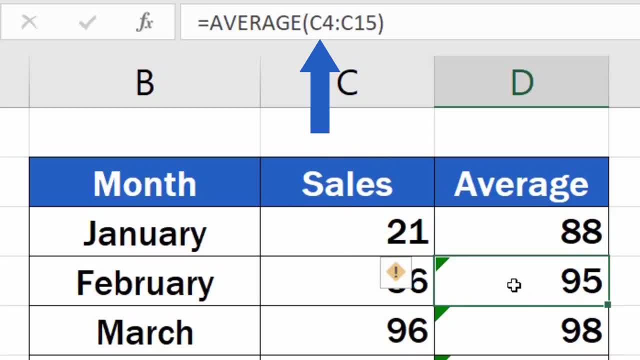 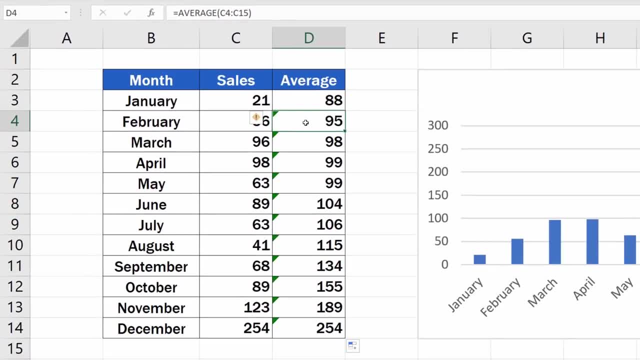 but in row 4 the range shifted down by one, so we've got C4 to C15.. This, of course, is something that needs to be fixed. To ensure the function calculates the correct value in each row. we need to make sure that the formula refers to the same range in each row. 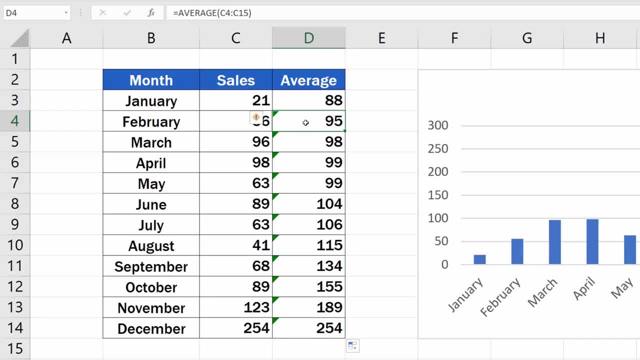 instance. so we need to anchor the references to the cells. let's click into cell d3 and pin the reference to the first point of the range c3. this can be easily done by clicking into the reference itself and then pressing the function key and f4. some of you might not need to press the function key this. 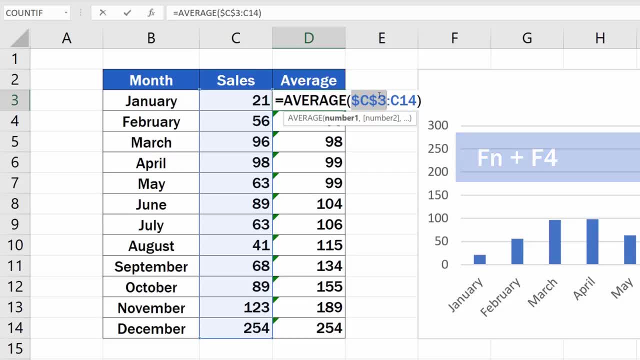 depends on what type of keyboard you've got on your computer. a dollar sign appeared right next to the letter and the number, which means that this reference has been fixed and it won't change. as we copy the formula in the rows below. every row will now refer to the cell c3. this is called an absolute. 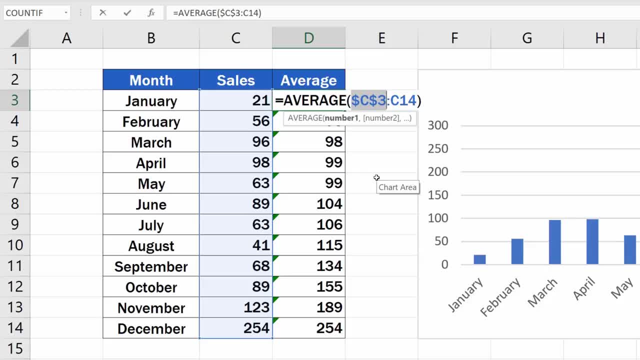 reference, as opposed to the so-called relative reference we had in our formula just a moment ago. let's do the same thing with c14. now, when the values have been fixed, we can press enter and copy the function to the rest of the rows in the column. 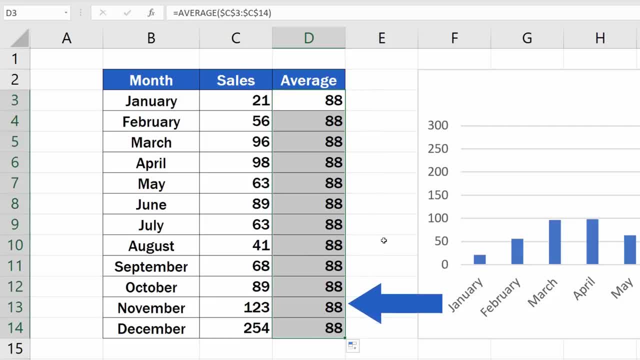 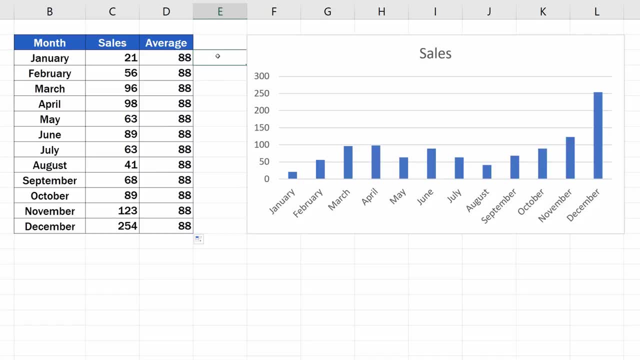 the result is now correct in each row, so we can carry on with adding the average line into our chart. but how do we do that? the easiest way to include the average value as a line into the chart is to click anywhere near the chart. the range of data already displayed in the chart has been highlighted in the table. 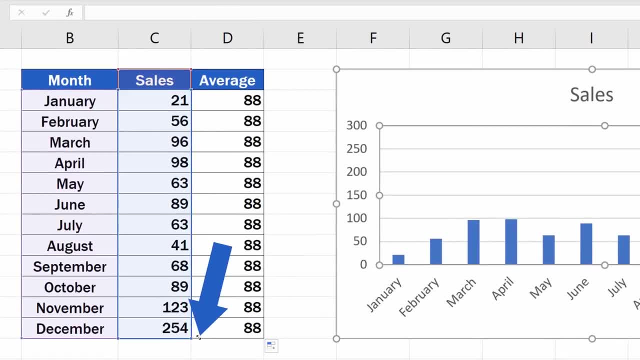 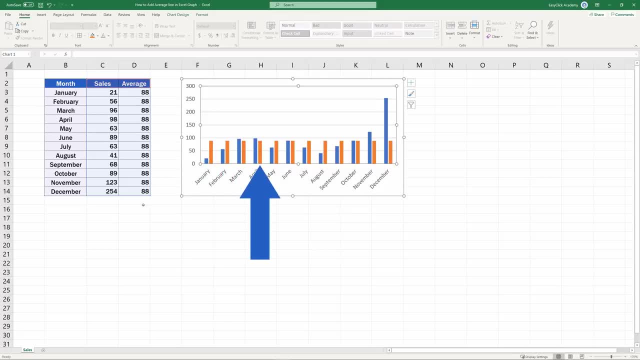 click and drag the bottom right corner of the selection to expand it to the average column. you can see that Excel included the new data from the average column in the chart. it's still not perfect, though. the average value now shows as a bar next to the bar for every month, but we want it to be displayed as a horizontal line. 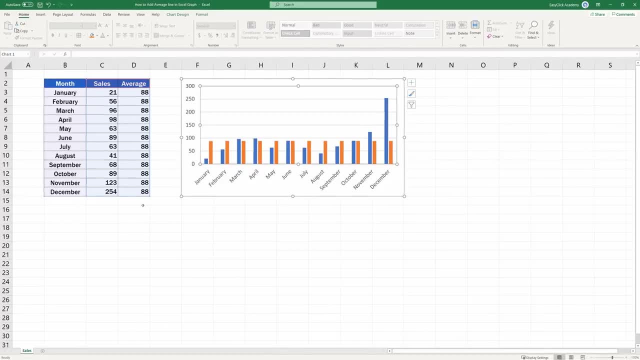 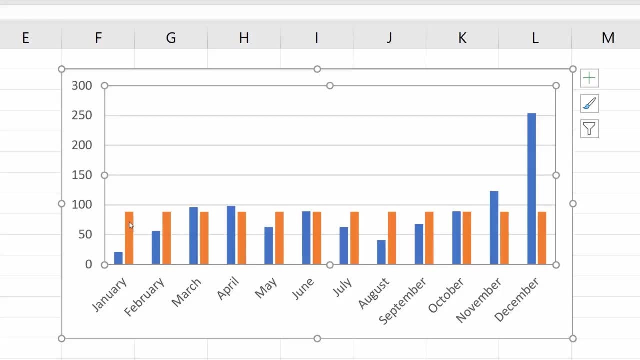 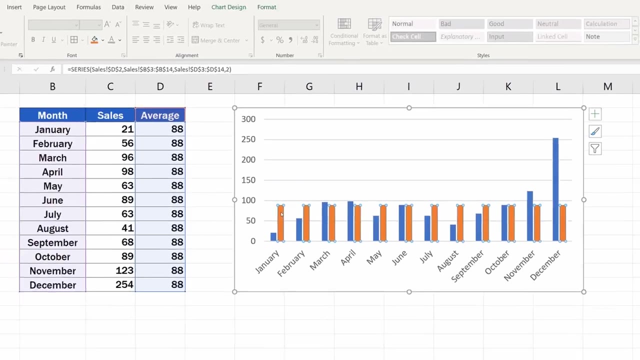 running through the graph. so let's fix this together to change the way the average data is displayed. click on any value from average in the chart. all values have been marked with these little blue circles. this means we can format them. let's click on the tab chart design here at the 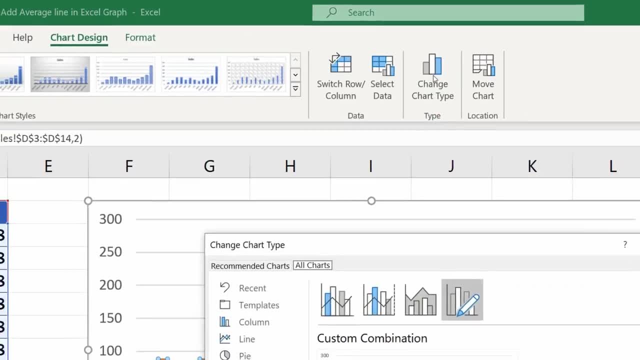 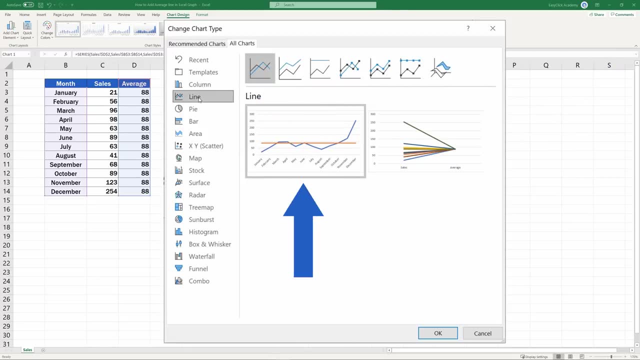 top and choose the option change charts type. it seems pretty straightforward here. we want a line, so we'll click on line. but watch out: if we actually clicked online, Excel would turn into a line graph- not only the average value but also the sales data. so both graphs would be line graphs and we want the sales. 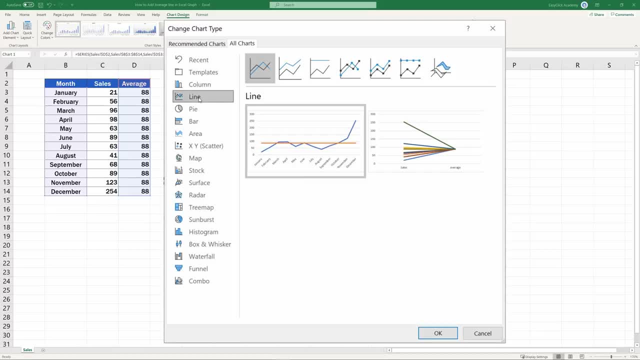 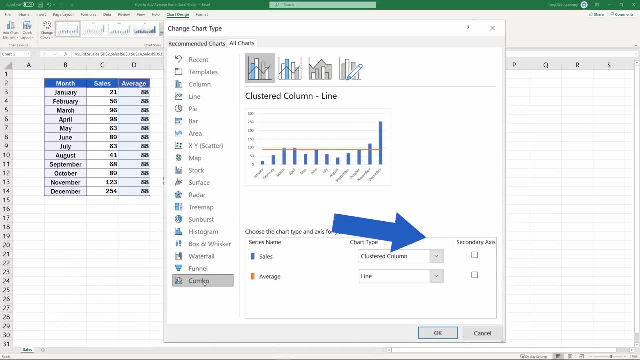 data to appear as they were in the original chart. that's why we need to combine two types of graphs, so we'll select the option combo. thanks to this option, we can select only the data from average to display as a line graph. the rest will stay as is and Excel will show the average value as a line. confirm.